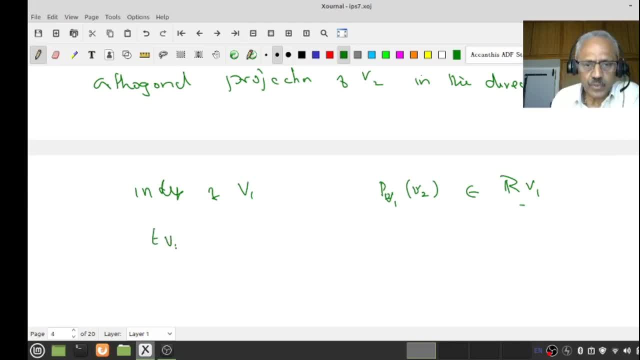 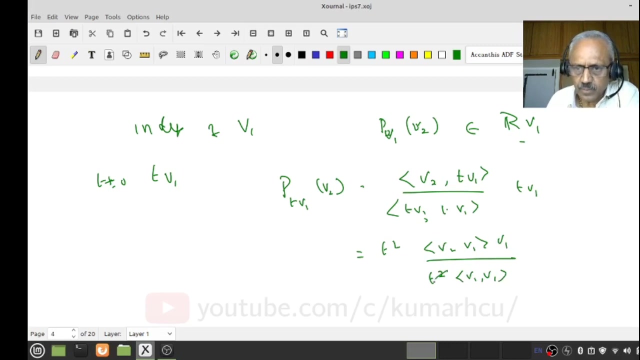 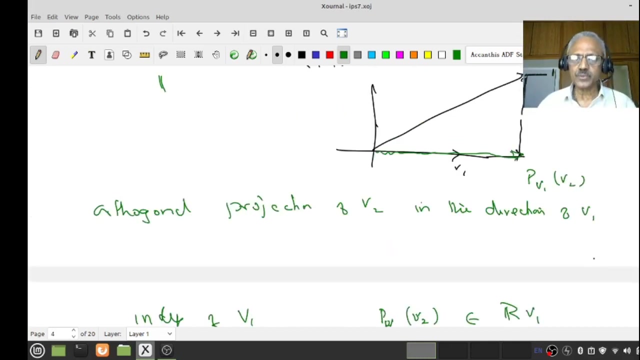 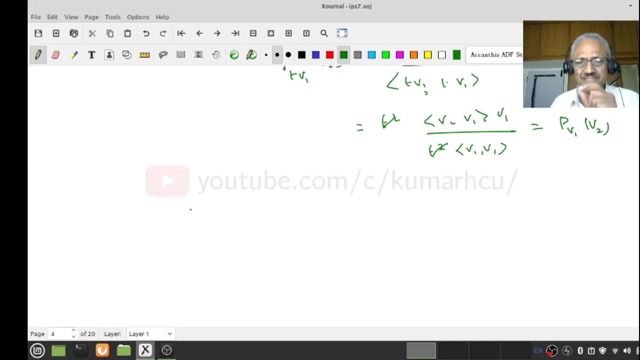 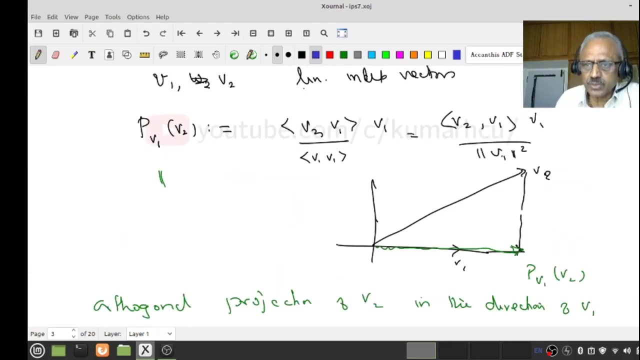 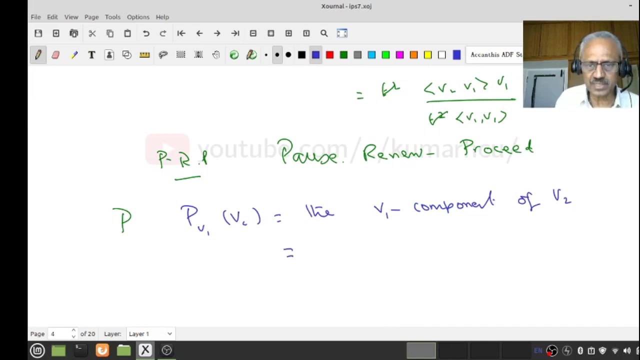 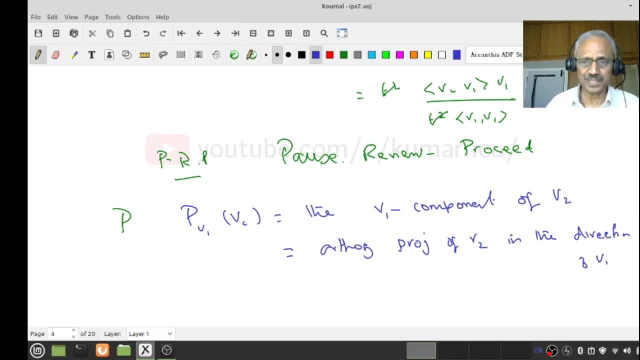 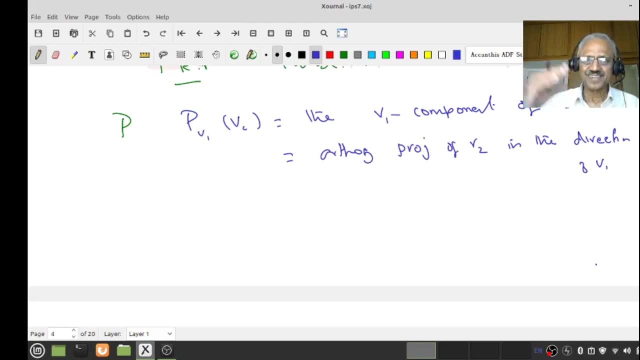 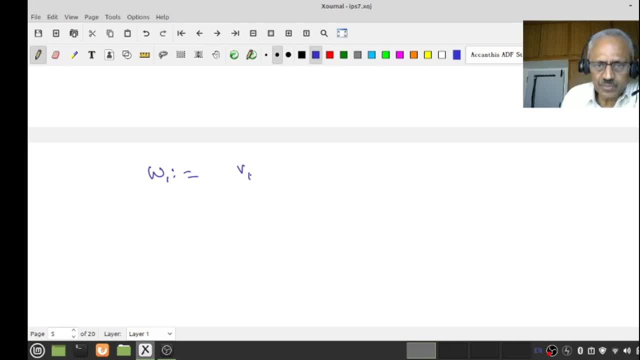 so let me call w1, keep the same notation as b1, w2 to be v2 minus orthogonal projection of v2 in the direction of v1, which is v2 minus inner product, v2, v1, v1 by norm, v1 squared, and what we found was this: w1 and w2 are orthogonal to each other. 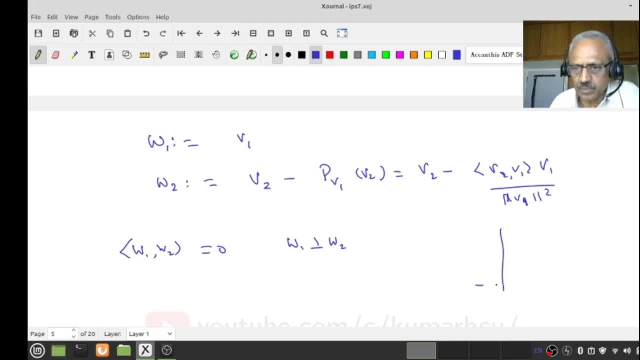 or perpendicular to each other. therefore, this again picture: this is my v1, this is my v2, this is my, this is my p, v1 of v2 and this object: okay, this is your w2. and remember, v1 is same as w1. okay, the picture shows they are orthogonal. we already explained. 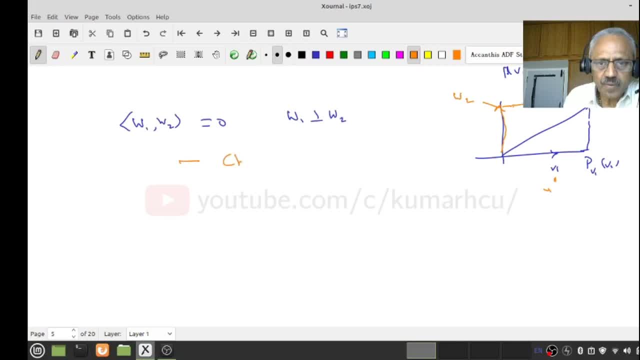 in the last lecture. but please check it again. okay, do you remember? that's how i master. whenever i come you, i will not say, yes, i have checked it, so i don't want to do it. no, you check it again so that you become very comfortable. you also become fast in computing. okay, please check it, i will. 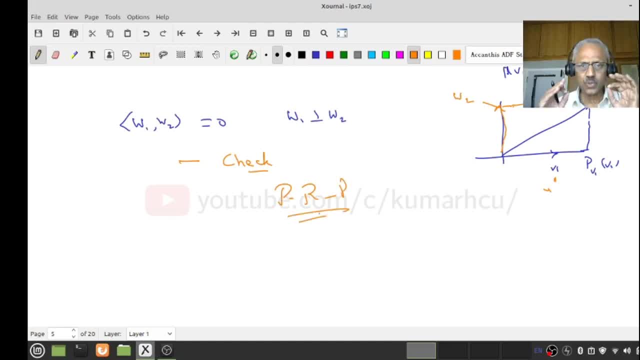 put a prp so that you feel comfortable. please do all these things. you will be master of inner product spaces, okay, so let us look at two things. so i started with v1 and v2 linearly independent, so i ended with w1- w2. then i found out w1 is orthogonal to w2 right now. notice that. can w2 be 0? 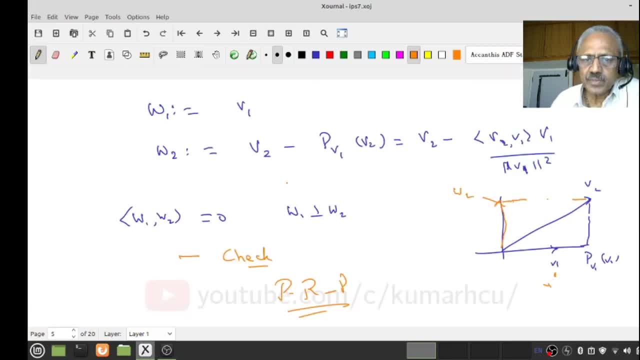 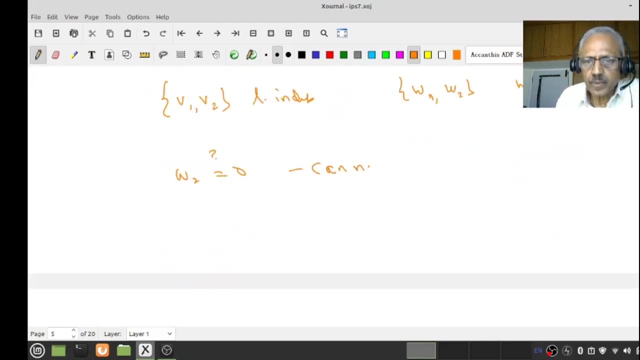 can it happen? suppose w2 is 0, what does it mean? look at this. that means v2 is a scalar multiple of v1, but that contradicts v1 and v2 are linearly independent. therefore, this cannot happen, right, because if this w2 equal to 0 implies v2 is a scalar multiple. 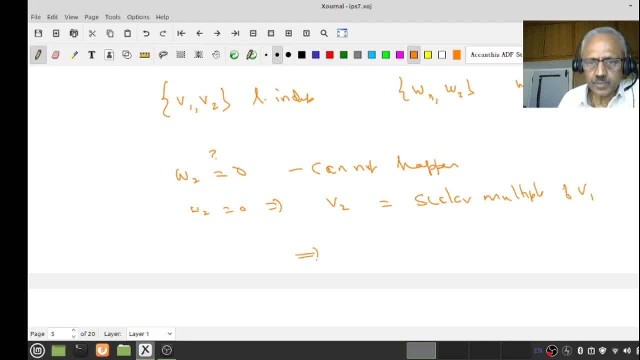 v1. therefore, this implies v1- v2 are linearly dependent. a contradiction, right? therefore, let us look at the subspace w which is span of v1 and v2. this is dimension of w is 2. right now, let us look at what is span of. 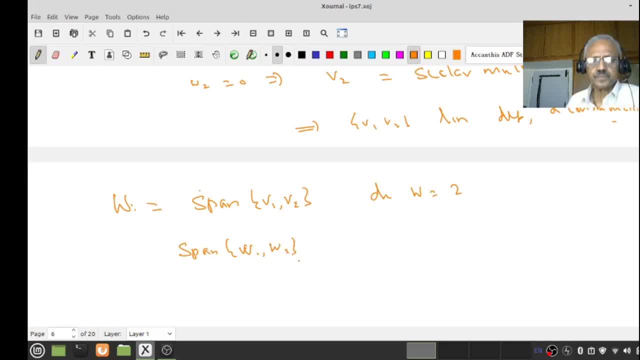 w1 and w2. right, i claim span of w1- w2 is same as span of v1- v2. right, let us go slow. okay, now what is the span of w1? these are the form a- w1 plus b- w2. but w1 is same as b1, therefore b- w2. but what is this? this is b times. what is w2? 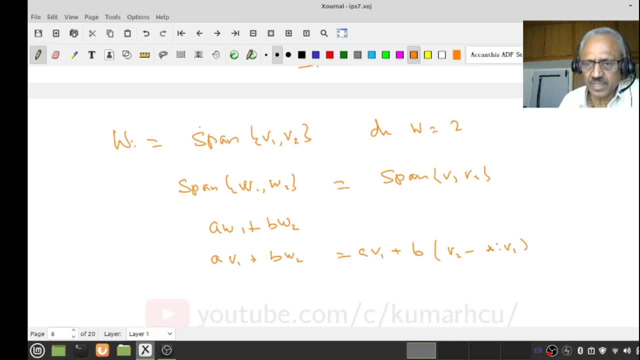 v2 minus some scalar multiple of v1. let us not worry about what the scalar. okay, the scalar may be b2, v1 by norm, v1 squared, etc. all right, this is v2, this is v1. okay, this is some scalar, if you want to call it, i mean, call it alpha, this alpha times v1. 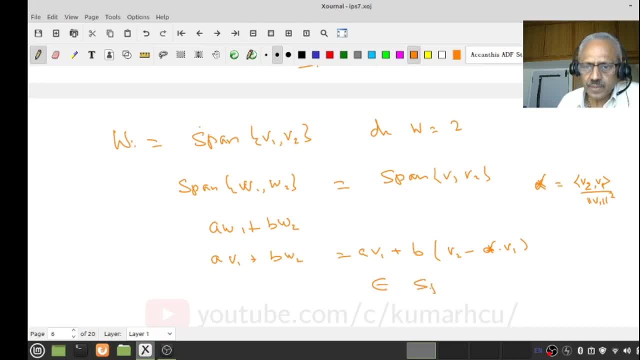 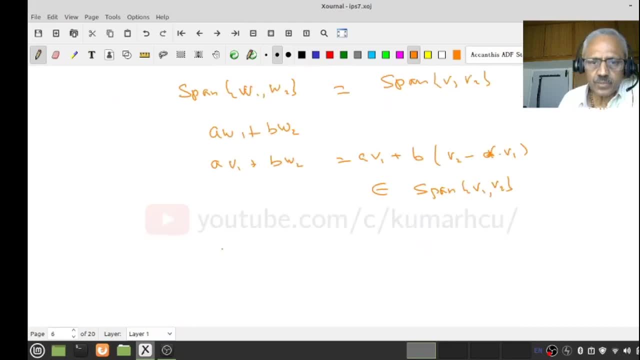 okay, therefore, this belongs to span of v1- v2. do you understand this? therefore, what is the conclusion? span of w1- w2 is containing span of v1- v2. okay, right now i claim w1 and w2 are okay, orthogonal to each other. that implies w1- w2 is 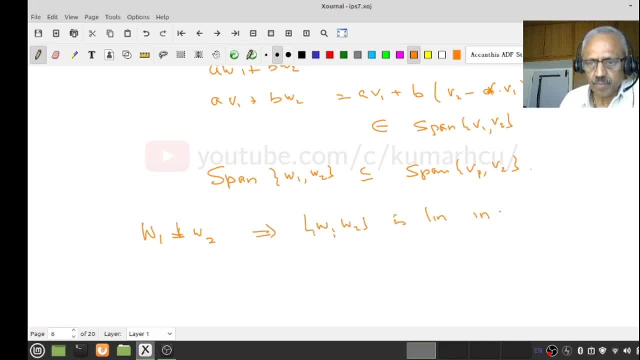 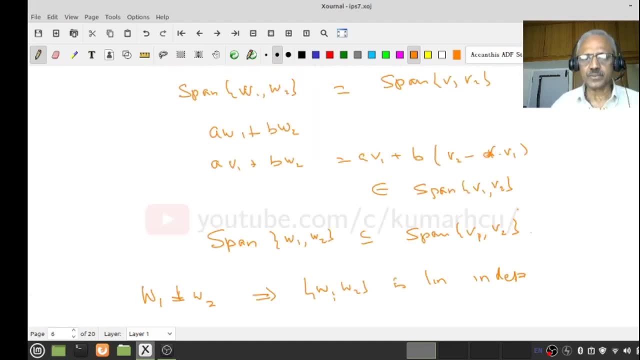 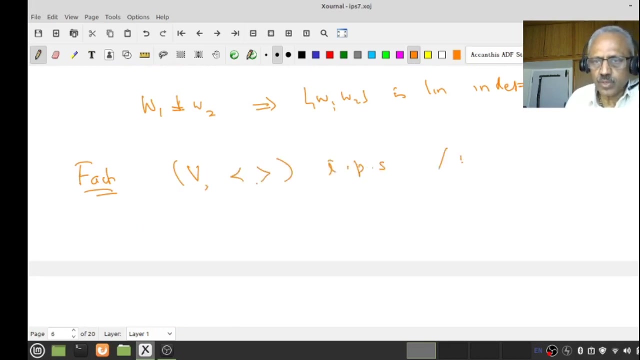 linearly independent. okay, why? this is a very, very general fact, but you can actually show that. okay, i will prove that. okay, let us make a very general fact. suppose v, this is an inner product space. okay, this could be over r, r, over c. and let us look at the set. okay, something like. 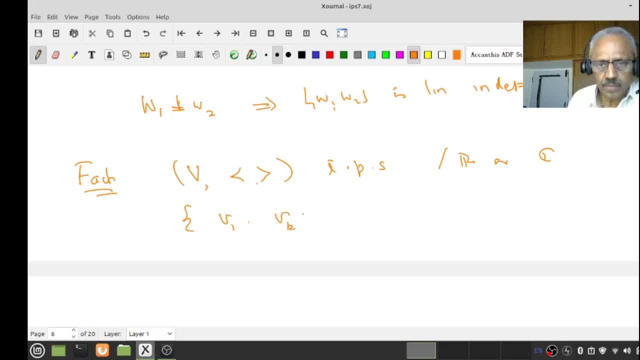 a v1. i might be able to help you if you finish your sentence okay. okay, this is a subset of non-zero vectors, that is, each va is not equal to zero. one angle right further. assume that v i intersection inner product, v j is zero or i n j. that is. this set is okay. call this set ss. 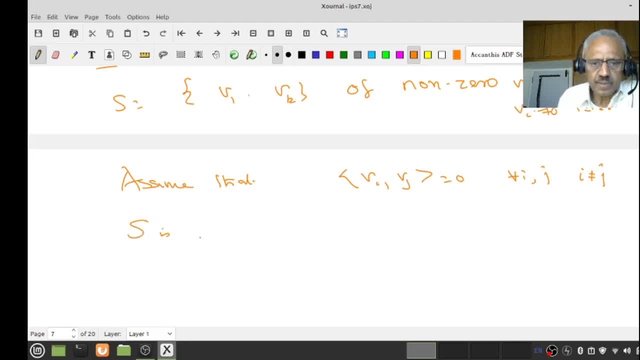 right, that means it's. one says s is a set of pairwise orthogonal, non-zero vector, right? so each v i is perpendicular to v, j per j naught equal to i, that's it okay. and each v is non-zero, all right, okay, then we claim s is. 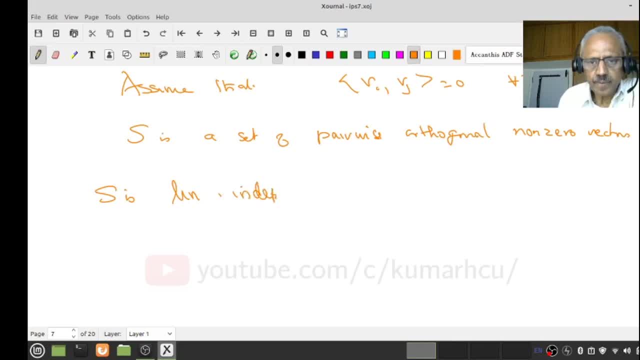 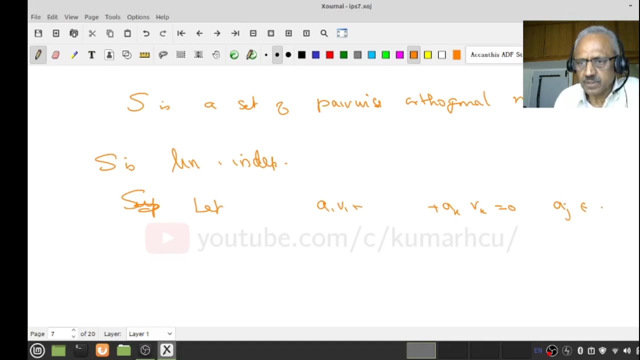 linearly independent? okay, so suppose not. okay, let okay, a, 1 v 1 plus ak, v, k, equal to zero where aj's are either in R or in C. right, okay then what do I want to prove? we want to prove each j aj is 0, this is what we want to prove. okay, now we have to use the 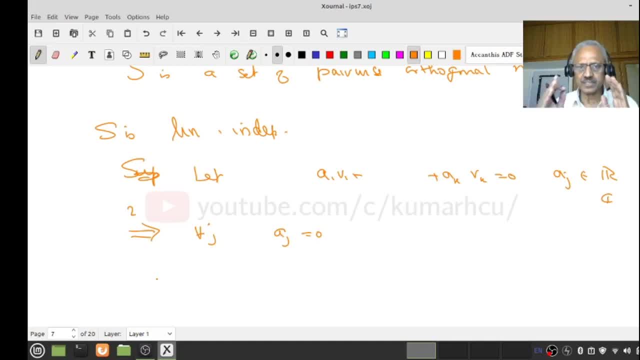 inner product, that is, by taking the left hand side, that is, a1, v1 plus a2, v2 plus ak, vk. okay, take the inner product of this vector with some vector so that I should get only essentially aj. the rest of them should be killed, the rest of them should. 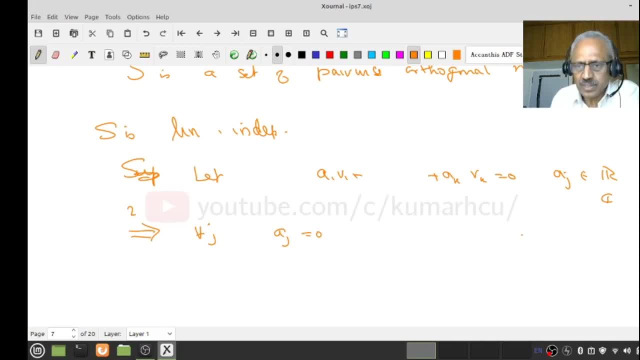 be. do that. you understand that. so I am looking for some vector v so that summation aj, vj, inner product v should be some scalar times, only some aj should come right or simply say ak should come, this is k. therefore it means just ar okay for 1, less than or. 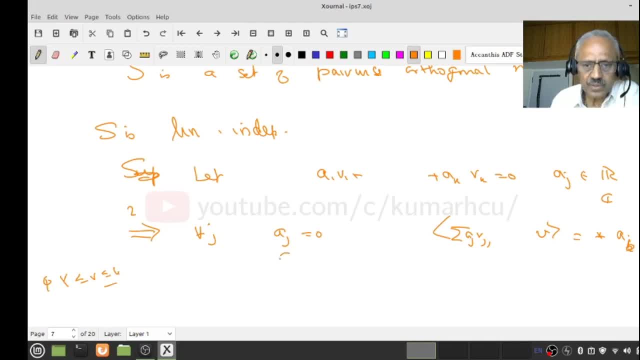 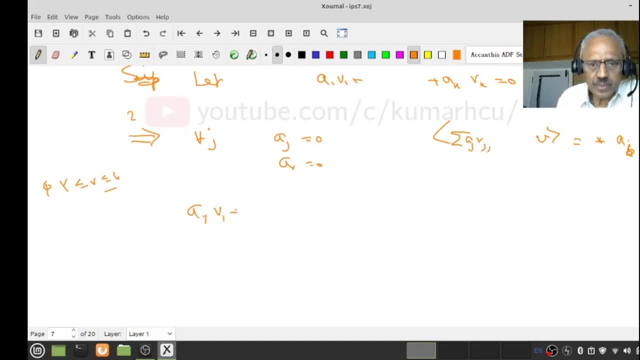 equal to r. That's very easy because if I take a1, v1 plus ak, vk inner product with vr, fix an r between 1 and k, then this will be a1, v1, vr plus ar, vr, vr plus ak, vk inner product. 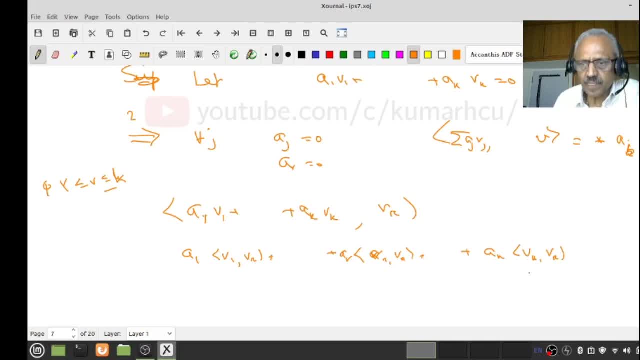 of this vector, right, but what do I know? okay, this is vr, vr. therefore, this is okay. this one will be 0, this one will be 0,. everything will be 0,, therefore, only surviving time will. 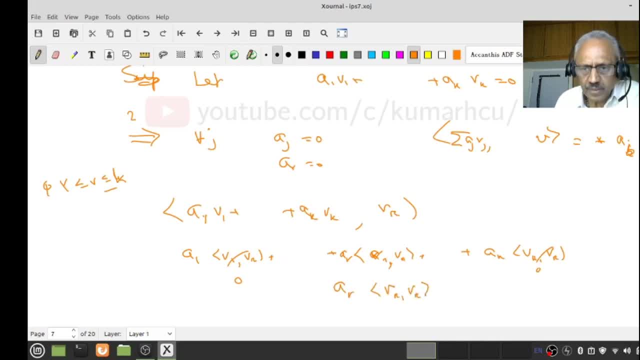 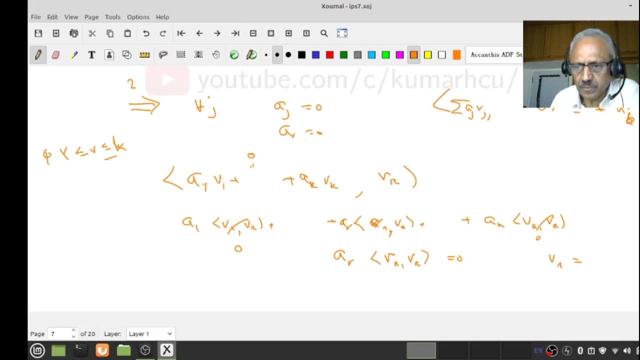 be ar into vr vr. that is equal to 0, because this object itself is 0, right, but what we know about vr? vr is not 0,. therefore, vr? vr is not 0,. therefore, this is not 0, right. 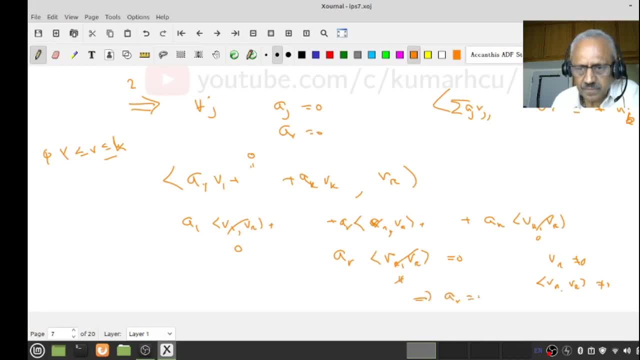 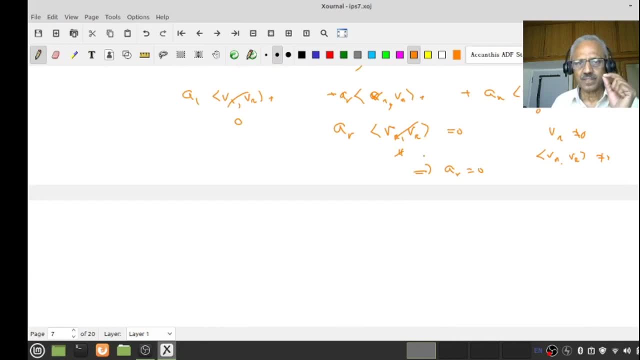 this implies ar is 0, right, so what have we shown? please go through the proof. the proof is very easy. okay, but don't try to memorize. what we are doing is we aren't using the inner product. so I am taking inner product of a1, v1 plus ak, vk with some vector. 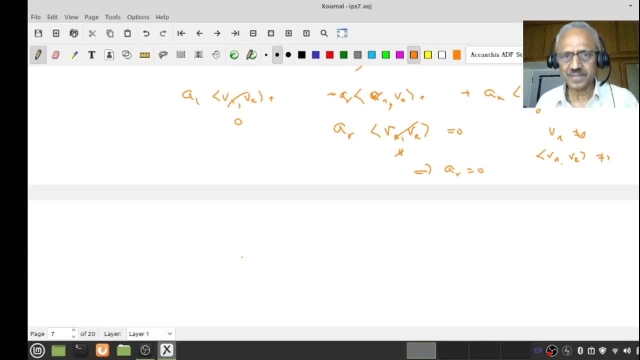 so that only essentially ar appears, since v1,, v2, vk are all mutually orthogonal. the obvious thing is: take inner product vr. therefore any vector is a1,, v2, vk, so that only essentially vi in the inner product vr will be 0,. if i is not equal to r, that is a trick, okay. 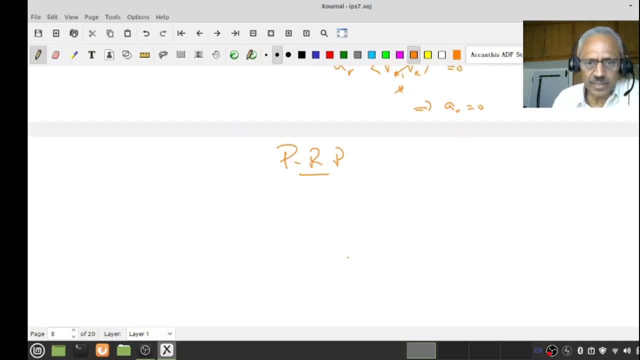 pause, review, proceed. so go back to our earlier situation. so w1, w2,- we know this is a non-zero, each one of them is a non-zero and they are orthogonal to each other. so, by the last fact, okay, w1, w2,. 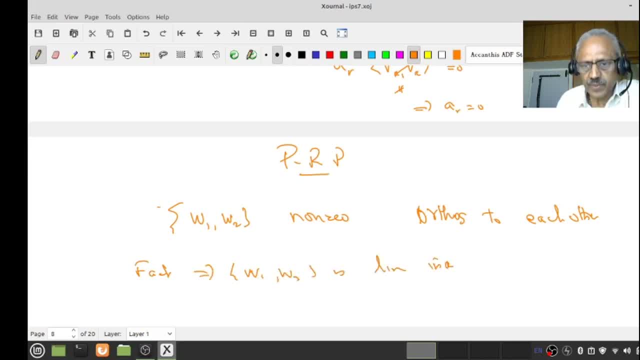 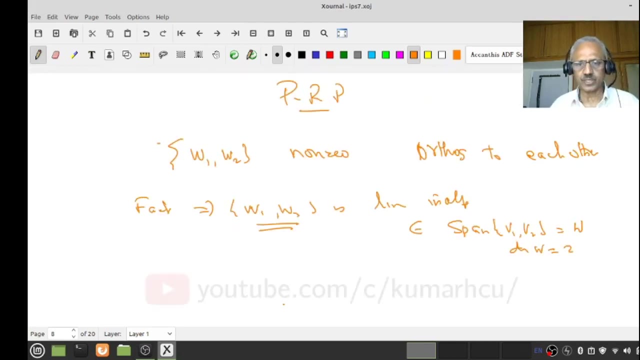 is linearly independent. and where do they live? they live in the span of v1, v2, which is w, and what is the dimension of w? 2, and therefore I have two linearly independent vectors in the vector subspace, two-dimensional vector subspace w. therefore, what do we know? 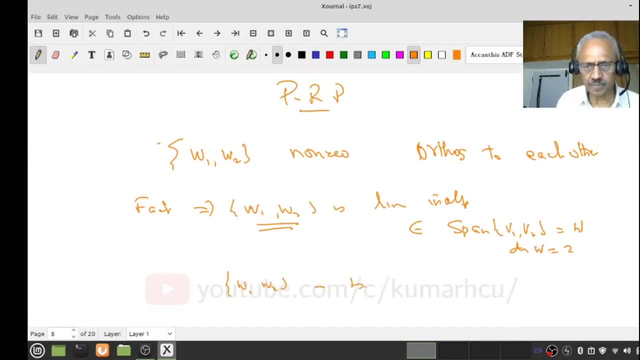 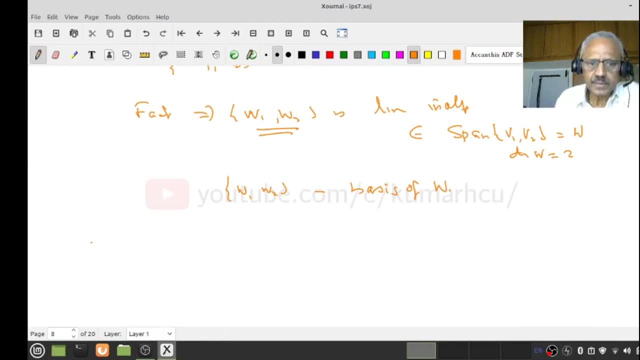 about this: w1, w2 is a basis, right? so let us summarize what we have done. let me just make sure that I have started in the thing. yeah, so what you have done is w with v1, v2 is a basis for w. maybe, if you want, take v itself this. 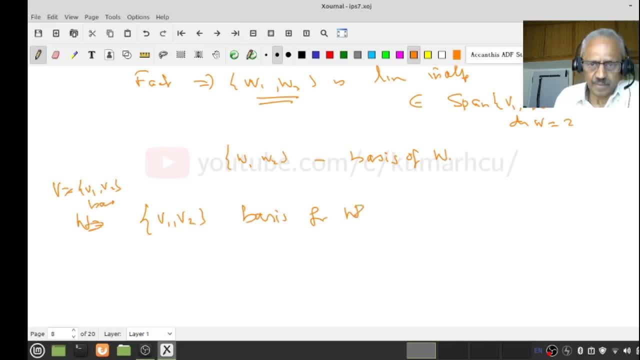 is a basis for: okay, this, okay. then out of this we constructed w1, w2, and then we have a basis. this is also a basis, but what is the important thing, it is an orthogonal basis. what do I mean by orthogonal? the set is orthogonal. set of non-zero vectors: okay. 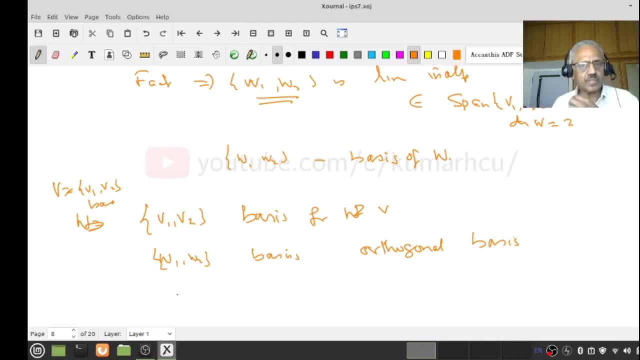 that means each other. any pair of vectors are mutually perpendicular to each other. okay, take wi and wj in this and i not equal to 0, wi intersection, sorry, inner product wj is 0, that is why we have proved yeah. 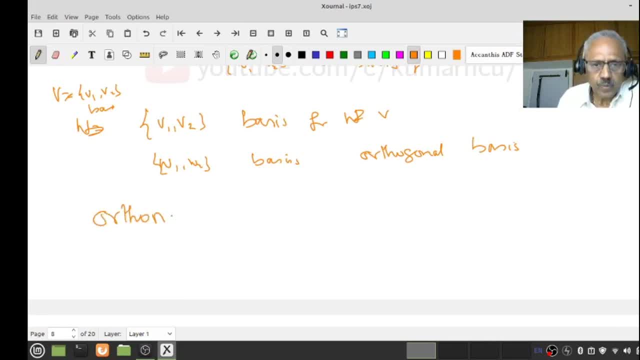 one talks about orthonormal basis is something like w, let us say u1,, u2,, so that this is orthogonal basis. okay, that means it is an orthogonal set and it is also a basis so that each of the vector is of norm 1, that is your normalizing each one of them will. 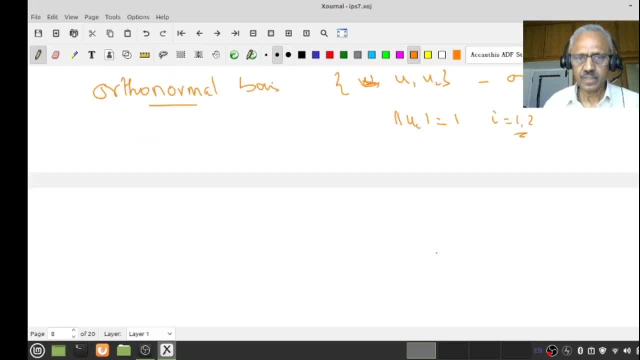 have same length. Yes, same length. okay, now let us go back. so, given v a basis- v1, v2,- we constructed an orthogonal basis- w1, w2, but it is very easy to construct an orthonormal basis. how? 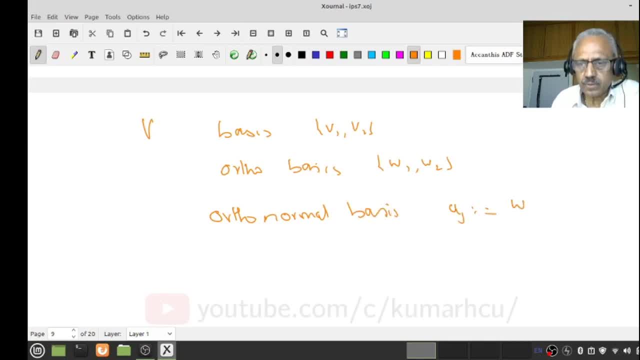 do I construct? put uj equal to wj by ram wj. Notice that this is w1, w2 are basic vectors from a basis. therefore, wj is not equal to 0 for all j. therefore wj by this. and what is norm of uj? this we had already done, maybe. 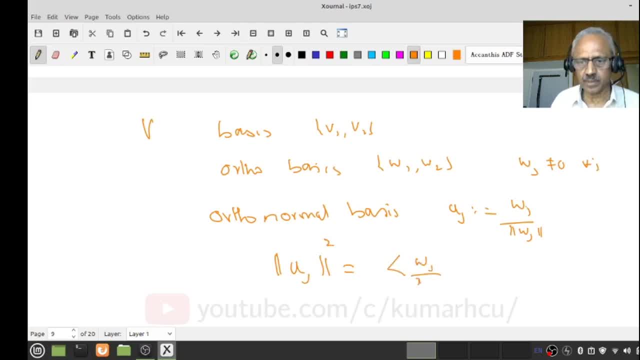 I have not done this. squared is okay: wj by norm wj, wj by norm wj. the scale has comes out. therefore, it is wj squared into inner product wj, wj. But this is norm wj, w2, therefore equal to 1, therefore, each one, one of the vectors. 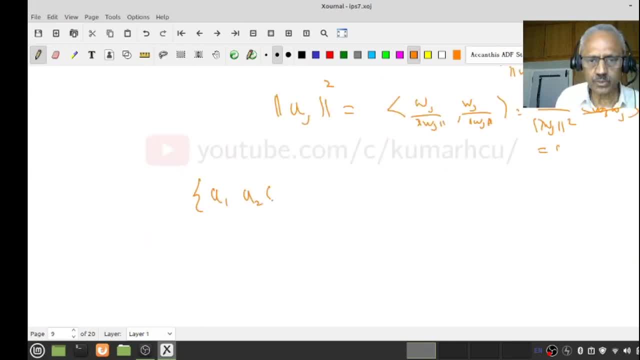 uj will be 1,. therefore, what I have got- u1, u2- is an orthonormal basis for v. that is it okay. pause, review- proceed. before I stop, I will just give an easy example. 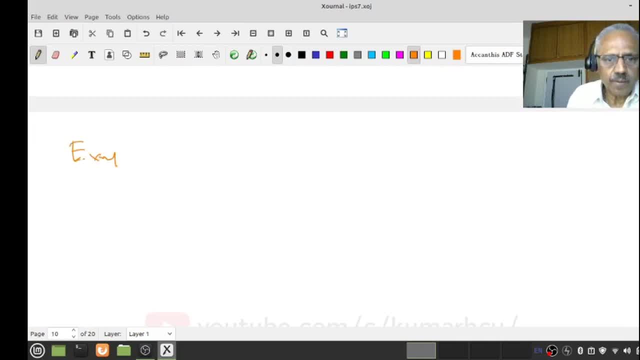 so that we will just quickly do that. Okay, let v be r2,. but the inner product, let us say it, is given by: let us say 2, 1, 1, 1, notice that 2 is positive, determinant is 2, 1, which is positive. therefore, we 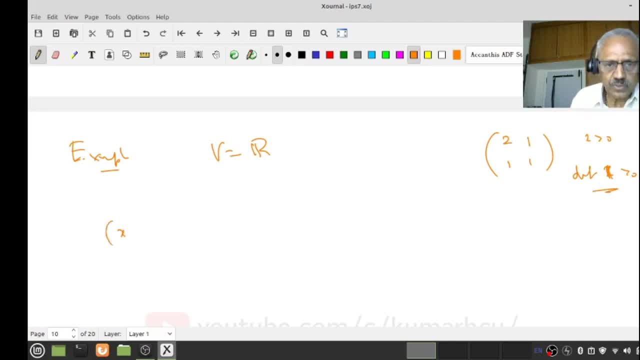 know this defines inner product. what is the inner product? suppose I have x1, x2,- sorry, x1, y1, inner product with x2, y2, this is given by 2, x1, y2.. 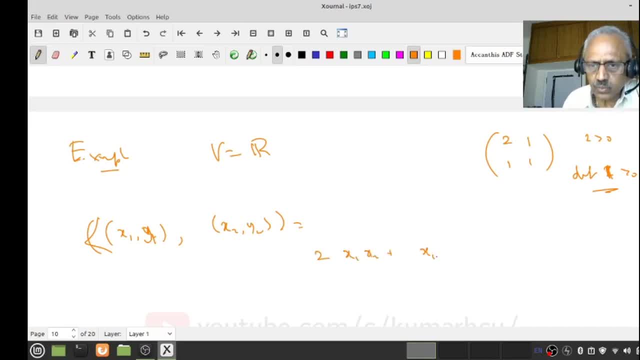 So I have x1, x2, plus 1, 1, therefore, it is x1, y2, plus x2, y1, plus y1, y2, this is the inner product. okay, and is it positive definite, therefore, if that is x1 equal to. 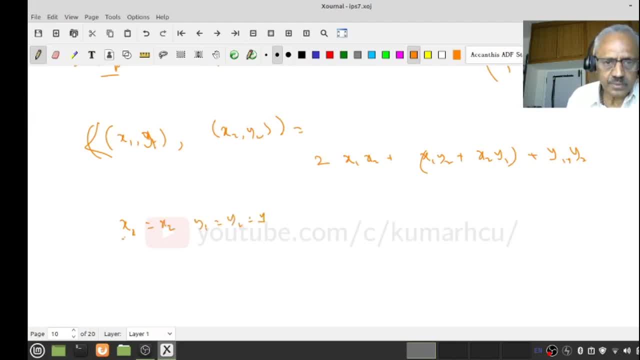 x2, y1 equal to y2 equal to y and this is equal to x, then inner product of xy with xy, y2.. So xy equal to 2x squared plus. this is x, xy, xy, therefore 2xy plus y squared right. 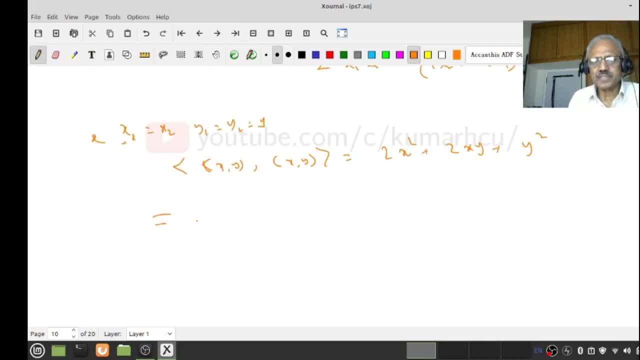 I am just doing it. okay, we did with the hb, but I asked you to look at something on your own. I am not sure how many of you did that. I know my students well. right, Therefore, to take out, then complete the square, that is, x squared plus xy plus y squared. 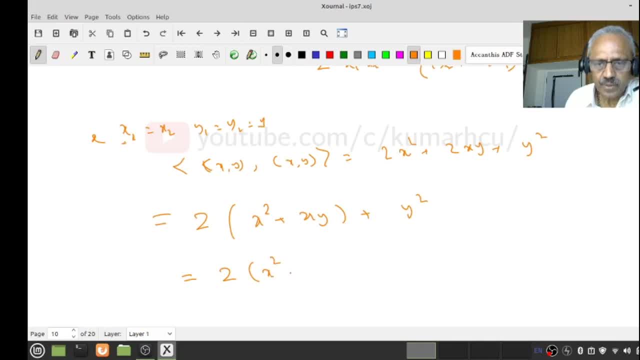 therefore this I can write as 2 into x, squared plus. how do I do that? So this is: you can write this as x plus half of y, whole squared, whole, squared, right, But this will be x squared plus 2 into x, into half of y, that is xy plus. I hope it. 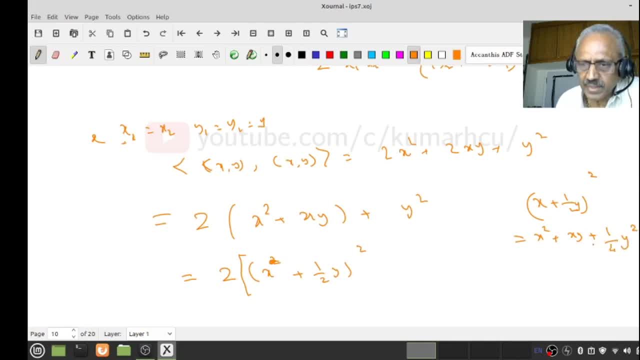 is 1.. So this is: you can write this as 2 into x squared plus y squared plus y squared, whole squared, right? I hope I am writing it correctly right? Therefore, x squared, this is xy, so I got xy, but this is extra. therefore, this is: 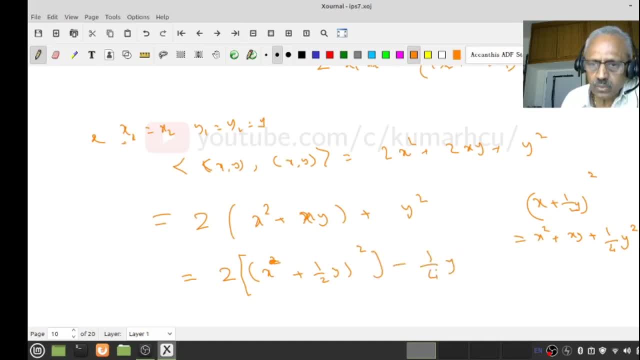 going to be minus 1. fourth, no, there is a 2 out, therefore 2 times right. Therefore, there is a 2 out, right? Therefore it is 2 times this plus y squared. So what do I get? 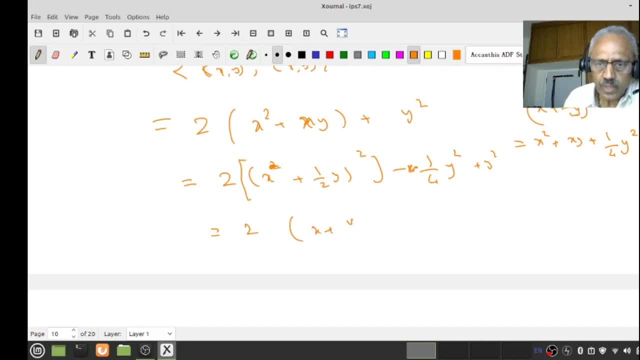 I get 2 times x plus y by 2 whole squared minus. This is half right, Therefore half of y squared plus okay, But this is equal to 0.. That means first thing is y is 0, because each one of the term must be 0,. therefore, 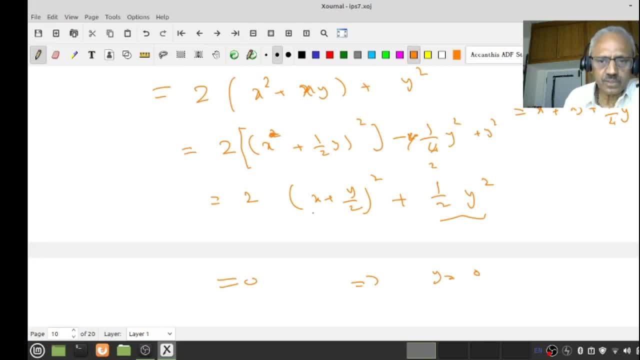 y is 0.. If y is 0,, that means 2x squared, because y is 0,, therefore 2x squared is 0,, therefore x squared is 0, and hence x is 0.. So this is positive definite. 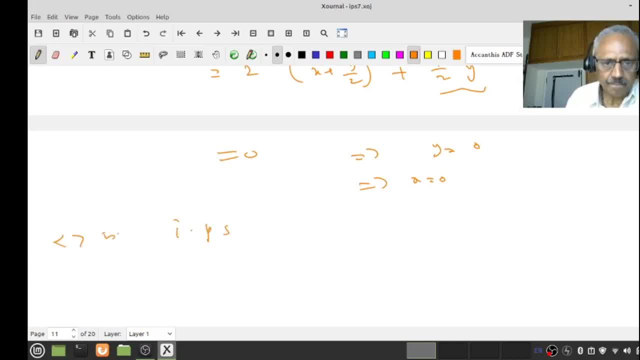 So this is an inner product. So this is an inner product. on R2, right Now, what is the? we can take my V1, V2 as a standard basis. E1, E2, right, Okay? 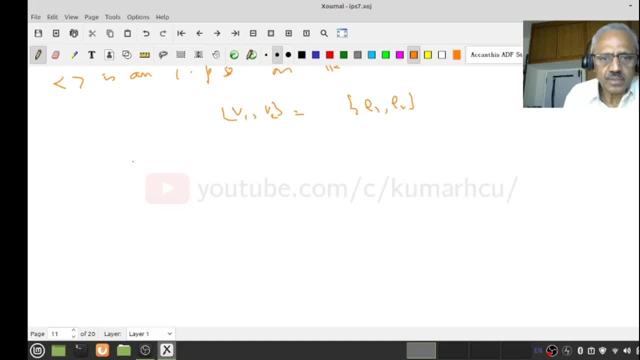 Now what is my W1?? So let us compute, okay. What is inner product E1, E1? This we know. just we have to go back to the definition that is going to be what for E1, which is 1,, 0,. therefore, x is 1, y is 0,. therefore, this will be 0, that will be. 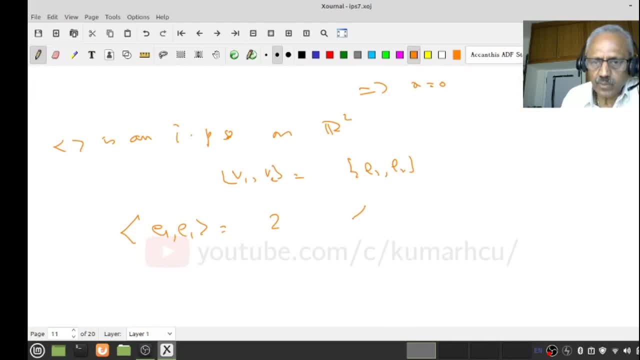 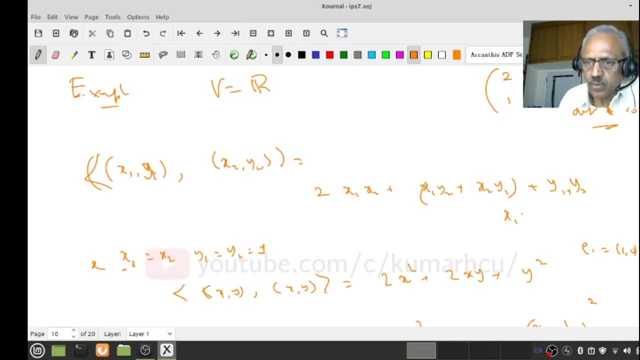 2,. therefore E1, E1 is 2.. And what is inner product E1, E2 with respect to this? Again, go to that. So this is my x1, y1,, that is 1, 0,. x2, y2,, which is 0, 1.. 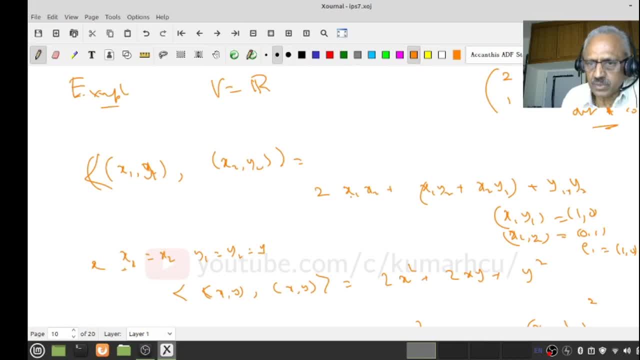 So substitute okay: x1, x2,, that is 0.. Then x1, y2,- that, That is 1, and x2, y1 are following. x1,- this is 1, y2,, that is 1, and x2 is okay then. 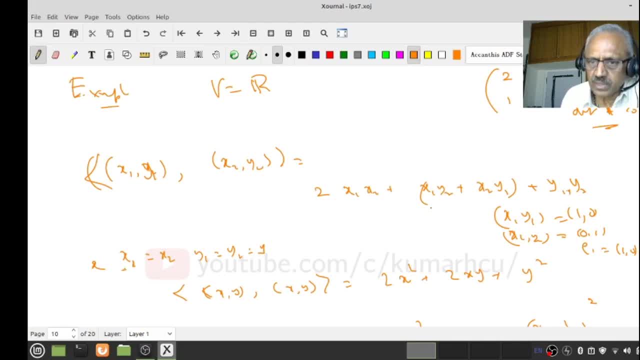 x2 times y1,, that is 0,. therefore, that is gives me only 1, and y1, y2, see, y1 is 0, y2 is 1,, therefore 0, okay, Make sure that you understand all this thing. therefore, it is 1, okay. 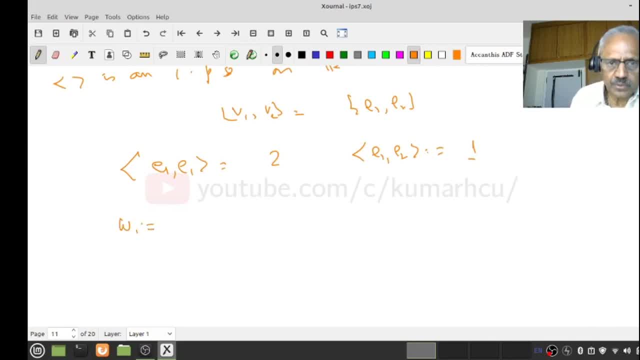 And I think now we know. So let we are going to take W1 equal to E1, and how do I check W2?? W2 will be E2 minus E2, inner product E1, and E1 and the length of E1,, that is length squared. 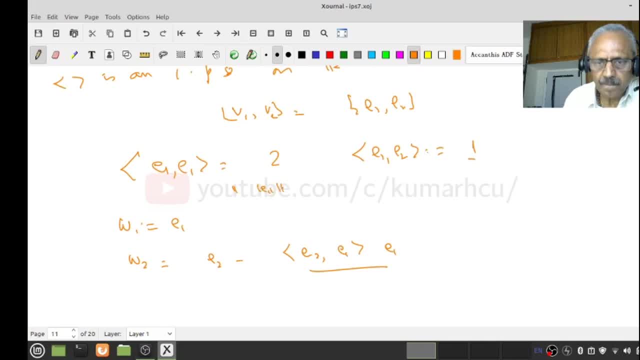 This is norm of E1 squared. okay, That is 2.. Are you following? But what is E2, E1?? This is 1, E2, E1 is 1,. therefore, I have 0, 1 minus. 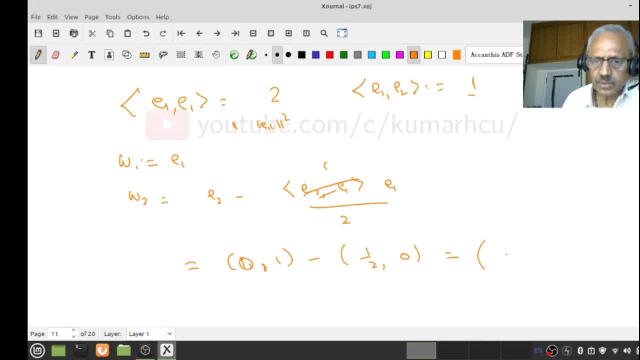 Half comma 0, that is going to be minus half comma 1, that is my W2.. So let us just make sure W1 is perpendicular to W2, therefore, what is my x1, x2?? So my x1, y1 is 1 comma 0, x2, y2 is minus half comma 1, and what is the inner product? 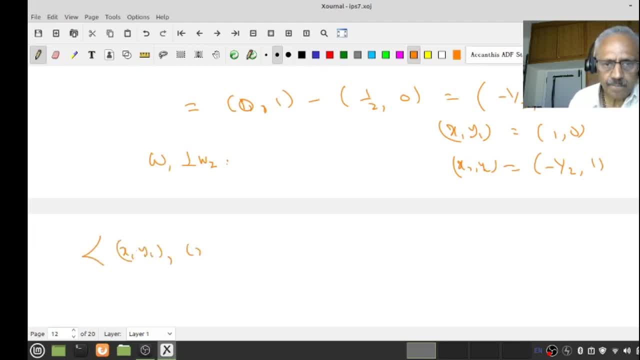 of those two things. So I have 2 times x1, x2 plus x1, y2 plus x2, y1 plus y1, y2.. See y1, y2, this is 0, and this is y2, this is 0, okay. 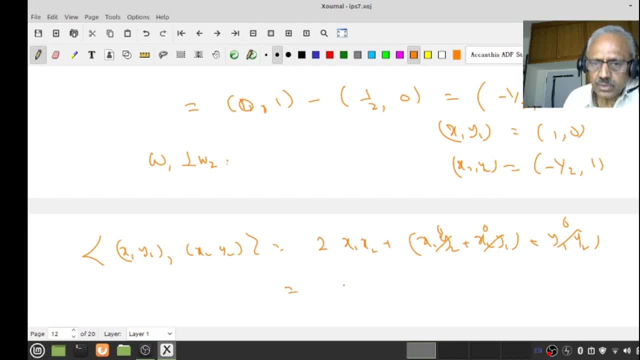 And this is x2,, this is 0, and x1, x2 is 2- into minus half. All right, So I do not seem to get 0,, so that means I made a mistake. yeah, Okay, let us do that.